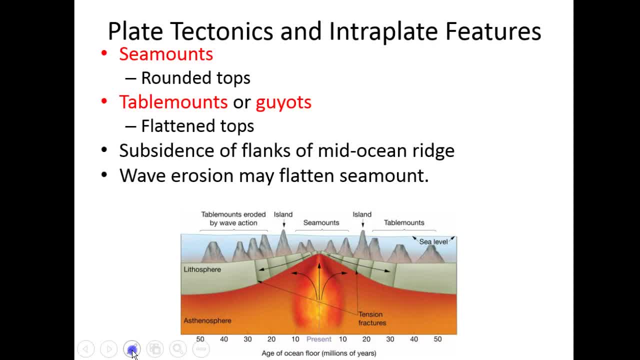 And so as these things are getting pushed up- let's see, as these things are getting pushed up along that hot spot, as they come up, as they continue to move outward, know that they're also kind of moving down, and so they need to be continually built in order for them to stay above the water, right? 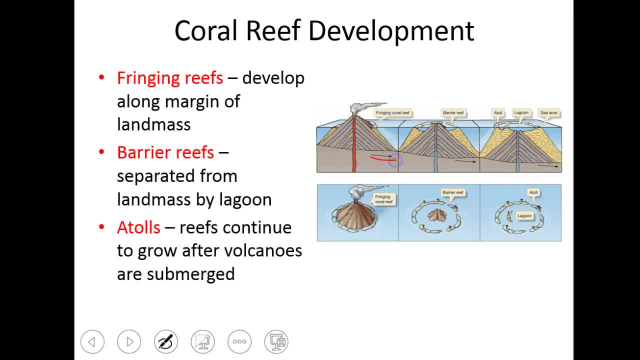 This kind of continually moving down, progression, of going to lower and lower sea levels is a really great way to build coral reefs. So we have fringing reefs and barrier reefs and atolls that are made from these, and so when this thing is an island like the island of Hawaii has a lot of coral reefs and it's a really great way to build coral reefs. 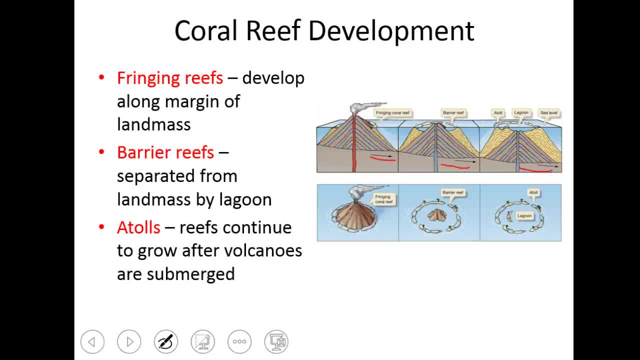 So we have lots and lots of fringing reefs. These are where coral animals kind of latch on to that substrate. It's nice and a happy region for them of warm, clear, nutrient-free waters that are not cloudy, and they're able to start that reef building process. 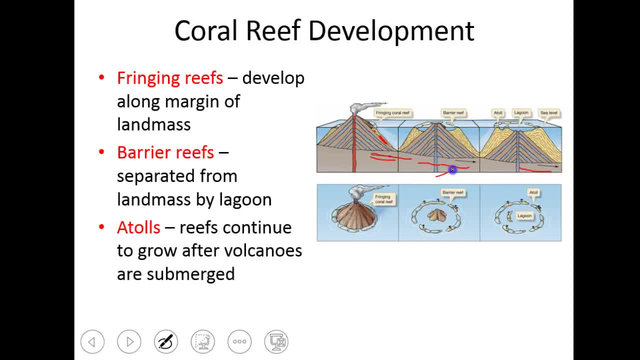 But as this island kind of slips along down into deeper and deeper water and maybe it gets eroded right and so we no longer have this big volcano that's getting cut off as it sinks down, it's a really great way to build a reef. 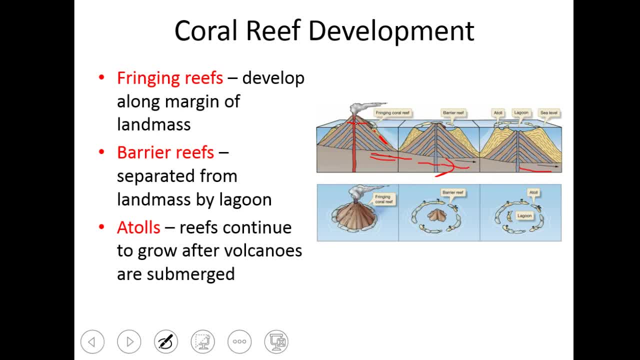 So as the reef sinks down and down, those reefs continue to build up and up and we get what we call barrier reefs, and so these are separated from that main landmass by a lagoon. The Great Barrier Reef is a really good example of this. 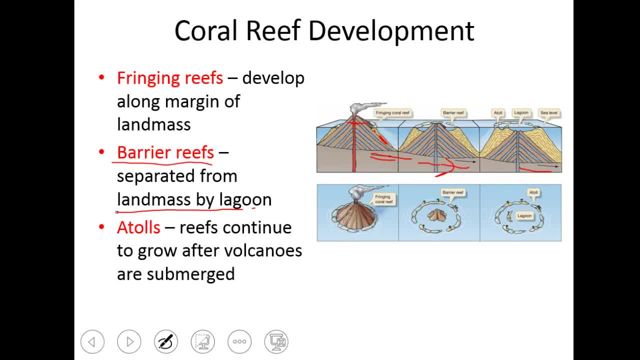 It's right offshore. And then, last but not least, is that island and what's now going to be a table mount continues to go down. Those coral animals are building on top of each other and we get basically just this: It's kind of a circular reef pattern where it used to be surrounding an island and we call that an atoll, and the reefs continue to grow even after that landmass is submerged and they just kind of start building on top of one another. 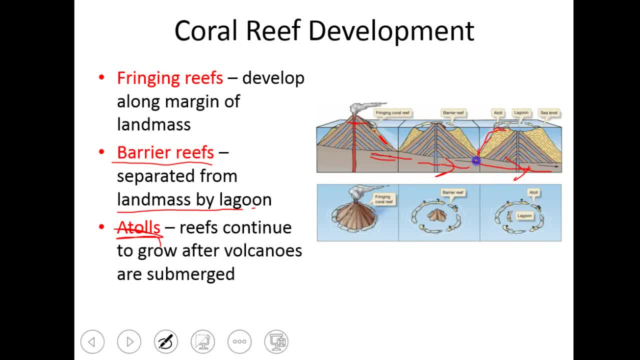 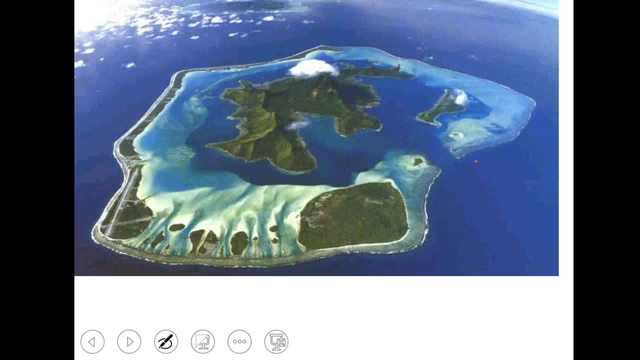 You can see how those coral animals are getting thicker and thicker and taller and taller so that they can stay at that nice happy level for coral. Bora Bora is a really great example of an atoll, So you can see where this volcanic island. 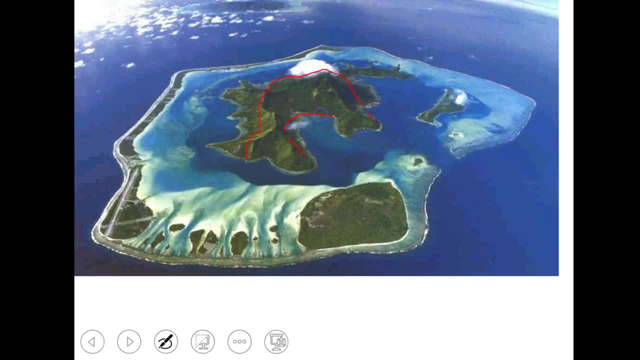 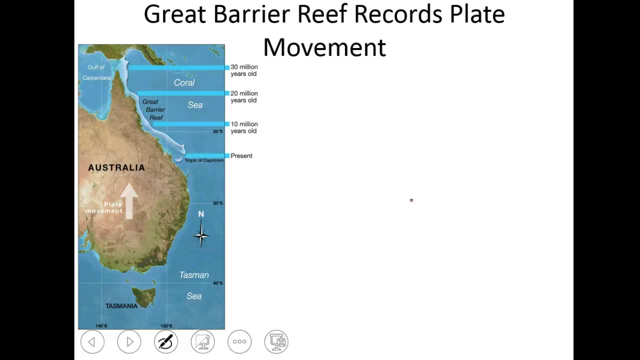 used to be and is subsiding right, and then all around it are what used to be fringing reefs and barrier reefs and have now become an atoll because they are so separated from that volcanic island. The Great Barrier Reef is a really good example, and I'm going to use the Great Barrier Reef as a platform to talk about how we also now know that plates move. 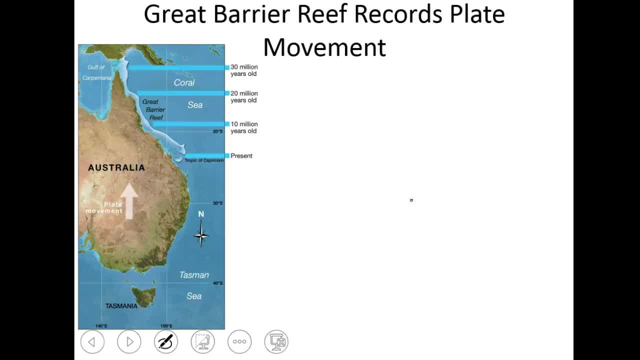 So we'll talk in a minute about the history, but this is a really good example. The Australian plate is moving northwest, and as it does so it's moving into warmer and warmer waters. So what used to be just on the threshold of happy coral warm water level 30 million years ago is now much, much higher, and that coral is still happy. 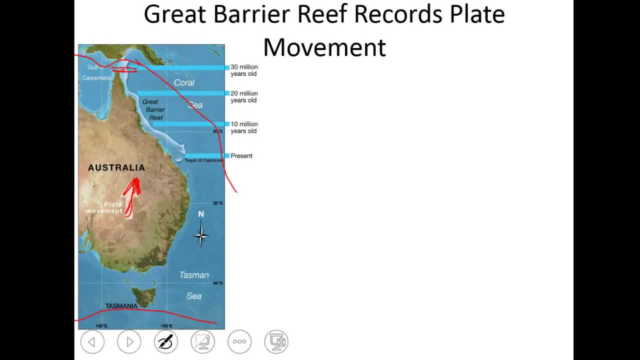 But as the Australian plate continues to move up, that Great Barrier Reef is able to expand downward as it moves up. And so as new parts of the continent pass that Tropic of Capricorn into the tropical region, then we begin to see reef development down, and down, and down. 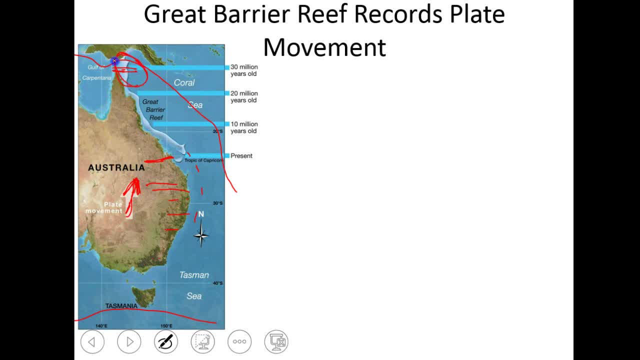 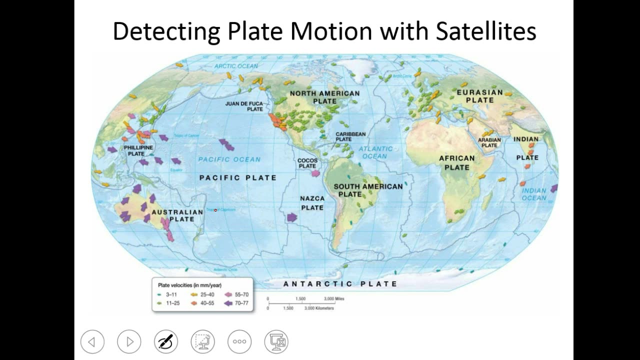 And so the oldest parts of the Great Barrier Reef are way up here and the youngest parts of the reef are down here and currently being built right along that tropical latitude 30 degrees south. Right Today we know that plates move Right. We've placed satellite receivers on all of these things and we can see the net direction and movement of the plates. 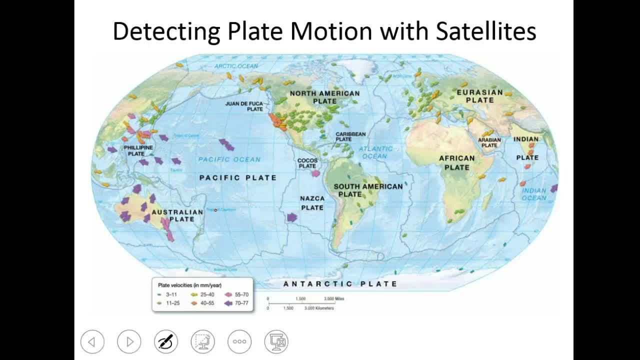 Right. Generally, the Pacific plate is moving northwest Very generally, Africa, the African plate is moving east. The Indian plate is moving northeast Right, And then The color of these arrows indicates how fast they're moving, And so what I want you to do is take a second and look and see which plate is moving the fastest based on this scale. 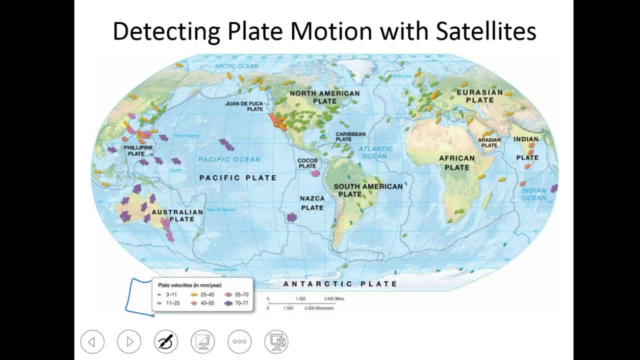 Come on. So, based on this scale, what we see in millimeters per year- And so remember, a millimeter is about the thickness of a fingernail- In millimeters per year, what plates are moving the fastest? And as I look, I see that this dark purple indicates. 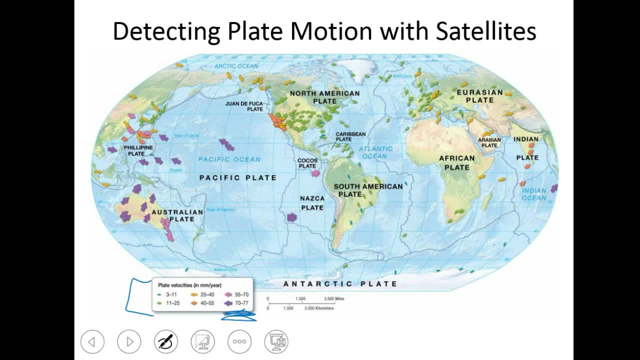 Moving the fastest. That's 70 to 77 millimeters a year. You can imagine that is about seven millimeters a year. So seven pinky fingers lined up. So we see that the Pacific plate and those Hawaiian islands are moving and growing. 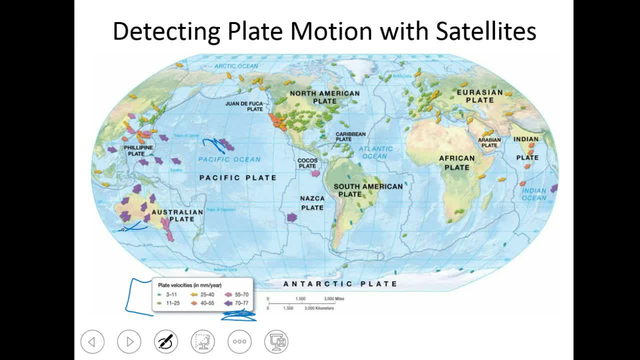 Australia is moving pretty fast And What else? The Nazca plate is moving pretty fast. That's where the Galapagos Islands are, a little hot spot out here off of South America, And so not all plate movement is created equal. When I told you the Atlantic is growing, that's actually one of the slower moving ones. 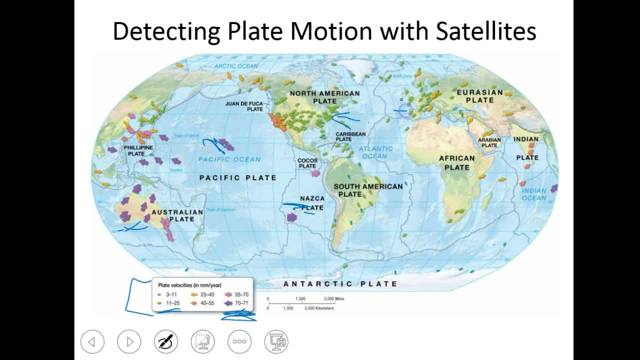 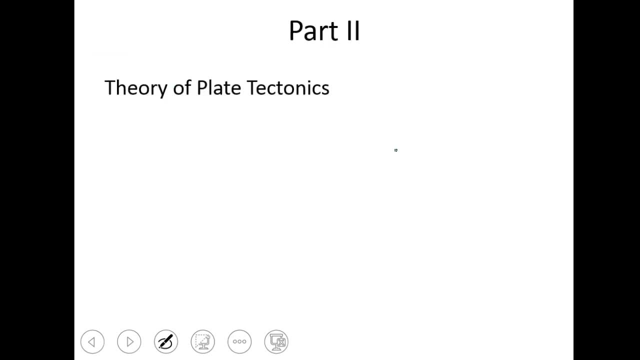 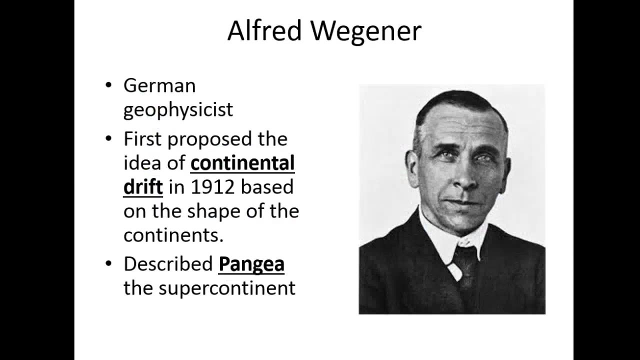 The North American plate is moving away here And the Eurasian plate moving away, African plate moving away, But all generally pretty slowly. So today we know that plates move, But this wasn't always the case. Alfred Wagner is a name that I want you to know. 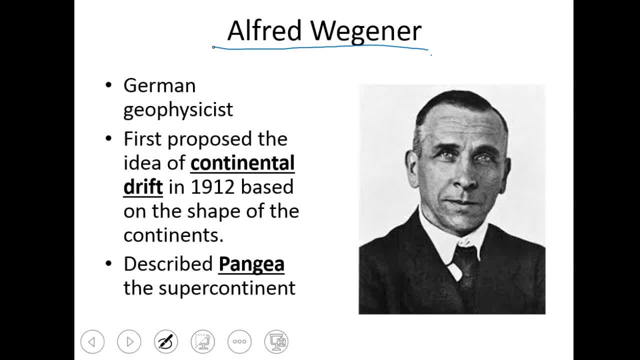 He was a German geophysicist, And he was the one that first proposed the idea of continental drift, what we know today called plate tectonics, And he proposed this in 1912, really early on. He based his ideas off of the shape of the continents. 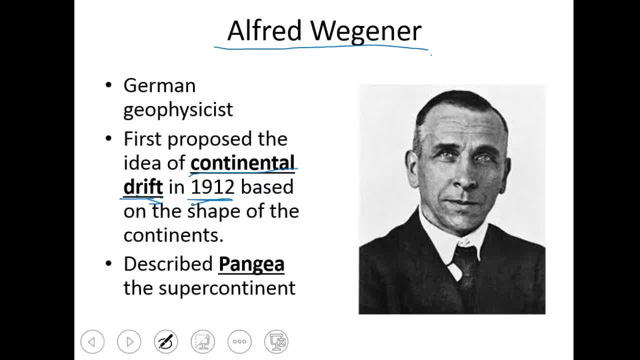 By looking at a map of the world he said: well, you know, it looks like South America pretty much fits into that little cove of Africa And that North America maybe could have attached on to Europe. And, you know, maybe Australia was up in the Arabian Sea now. 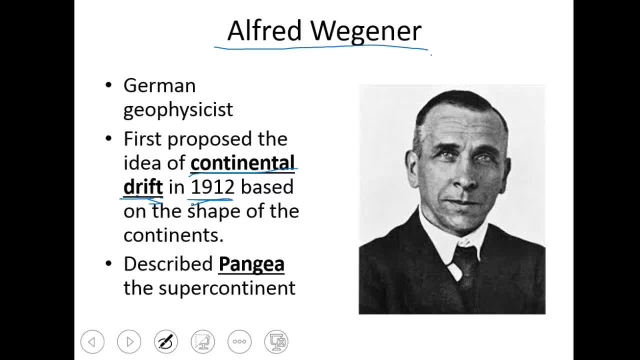 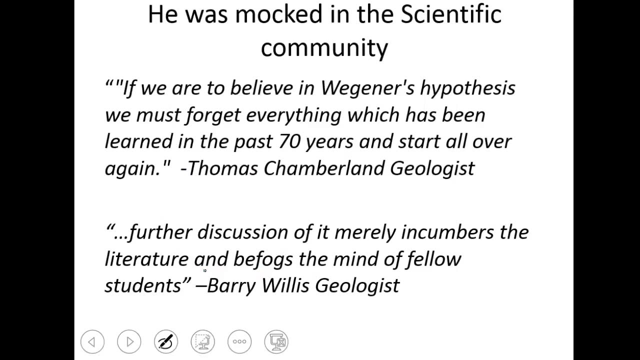 And so, just by looking at a map, he described Pangea, the supercontinent that, long, long ago, all of the world's land masses were this one supercontinent. When he presented this idea in 1912, he was completely mocked in the scientific community. 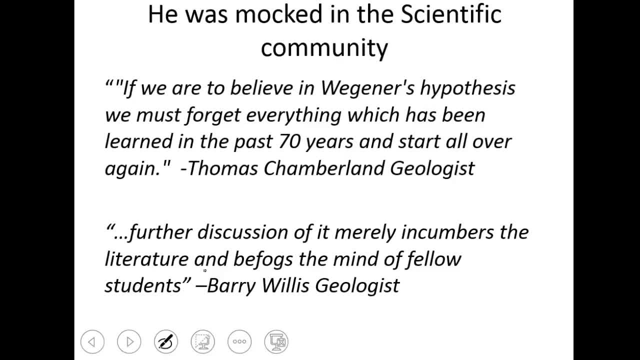 Nobody believed him. They thought he was full of malarkey. And he says: you know. so here's a couple of quotes against this. It says: if we are to believe in Wagner's hypothesis, we must forget everything which has been learned in the past 70 years and start all over again. 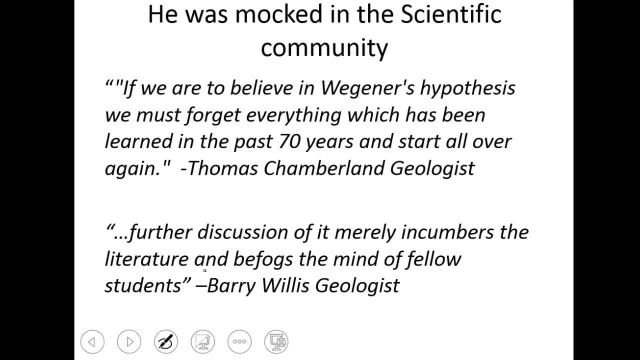 And further discussion of it merely encumbers the literature and befogs the mind of fellow students, And so people were saying this is so funny. So people were saying this is so preposterous. It would be like saying that everything that you've learned in your intro biology class was wrong. 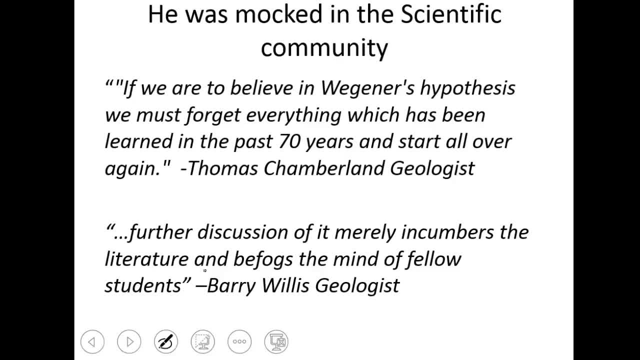 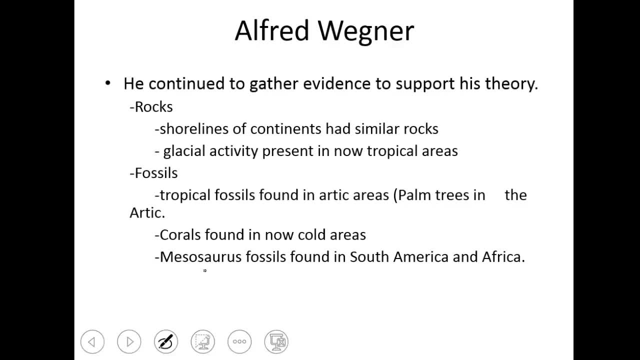 And this is a crazy idea and we can't teach it, So let's just throw it out. And they did, And he continued to gather evidence to support his theory. Ultimately, he was never recognized in his life for his work, But I do want you to know he's supporting evidence. 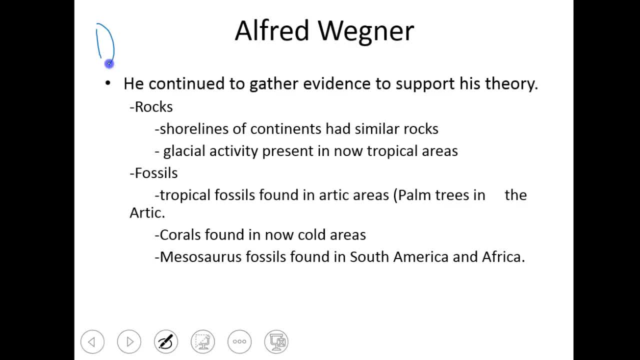 So Wagner's supporting evidence first and foremost was a continental fit. All the continents fit together And it just, I mean, it looks like a puzzle. It's been taken apart, And so that was his first kind of guess. But then, when people laughed him off the face of science, he continued to collect evidence. 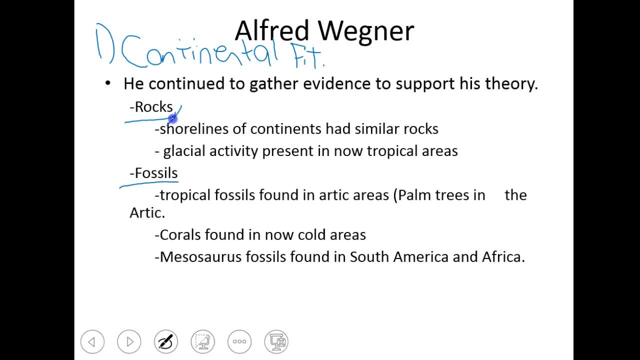 He collected evidence in rocks and fossils. The rocks that he found showed that the shorelines of the continents had similar rocks, And so he would look in the Appalachian Mountains And in European mountains And he would find similar rocks of similar ages. He would also see evidence of glacial activity, like ice- ice activity in what are now tropical islands. 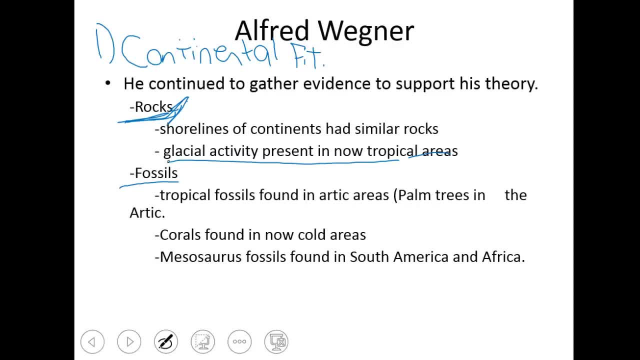 And that tells him that you know these are tropical now, but at one time they must have been somewhere else. He would see fossil evidence that tropical fossils are found in Arctic areas. For instance, down in the Arctic we are finding. 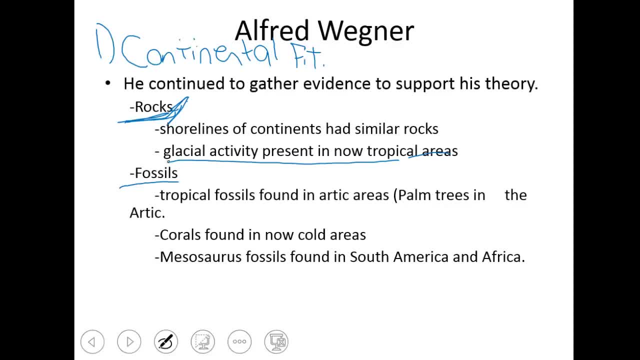 palm trees and corals and seashells from when it was not in a cold region of the world. We find corals now in cold regions of the world And then beyond just those like hmm, that's an odd animal for this place things. 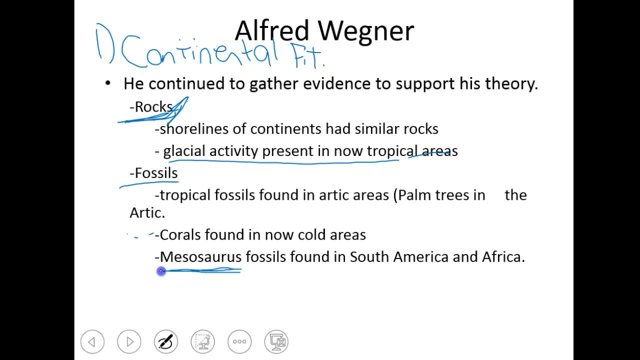 Mesosaurus fossils. These are an example of a fossil that's found in both South America and Africa and the southern portions of it, And so these mesosaurus fossils. you know, it's really unlikely that we would have the exact same animal develop on two continents that are so far apart. 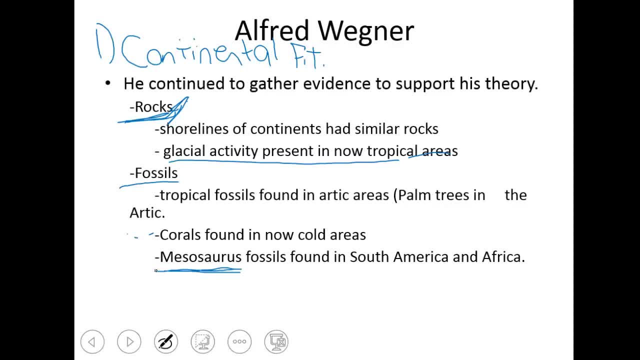 And so finding examples of plants and animals across what is now the Atlantic Ocean is a really big deal. They were the exact same and in the same kind of rocks, which is the idea that those continents used to be together, And so he had rock evidence. 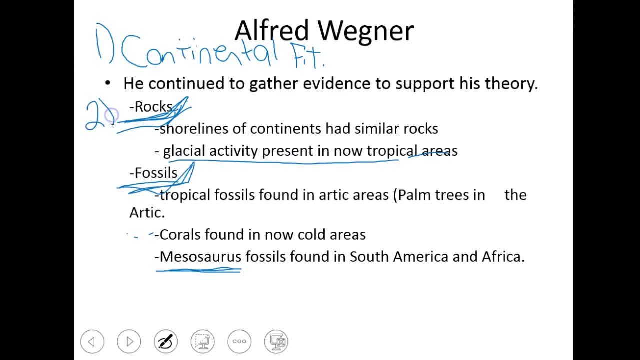 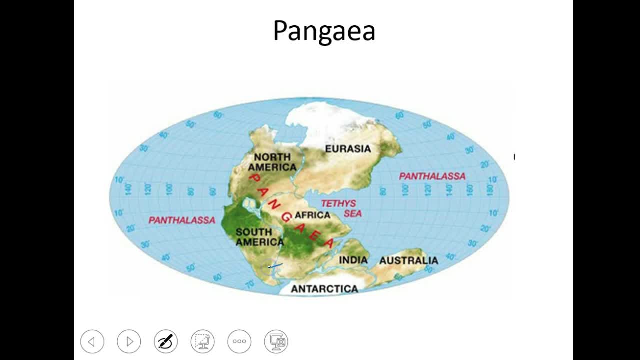 He had fossil evidence. There was continental fit Right That suggested this as well. And this is what he proposed: That South America was right next to Africa and that North America was right next to Eurasia, with Australia fitting in down here. Now what we see is that India kind of moves up to Eurasia. 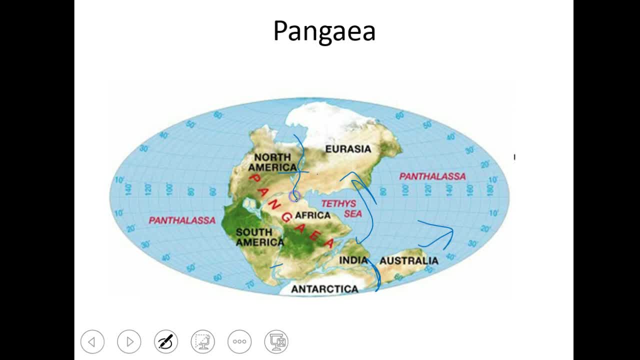 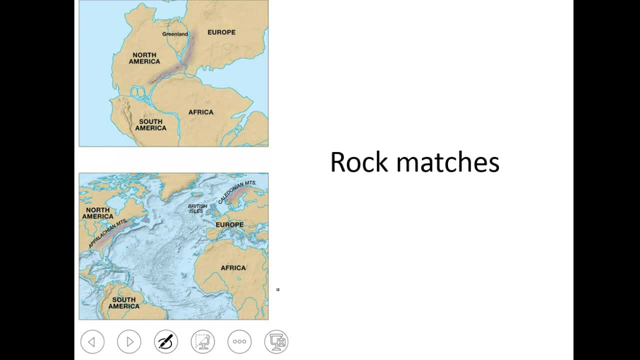 Australia moves this way. There was this rift valley developing here which would become the Atlantic Ocean, And here and here There we go. And so he would see the rock matches Right. The rocks in the Appalachian Mountains and the Caledonian Mountains are the same kinds of rocks. 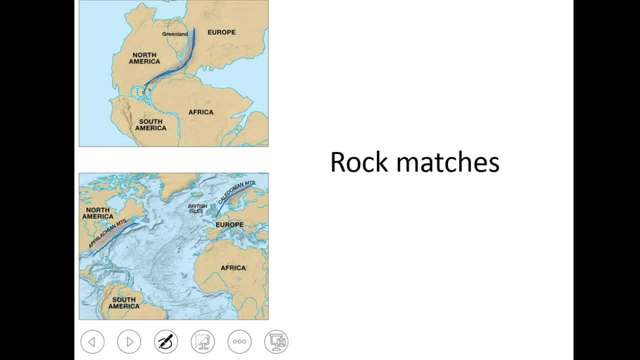 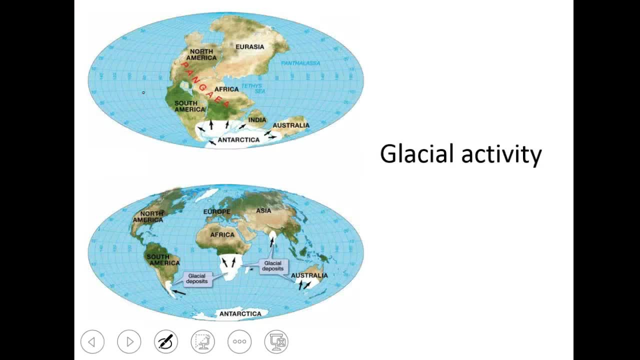 And that these formed when these were together. Right, They are. this one big continental, continental converging plate, creation of mountains. Right, He saw glacial activity in what are now warm places, And so South America, Africa, India and Australia all have evidence of glaciation. 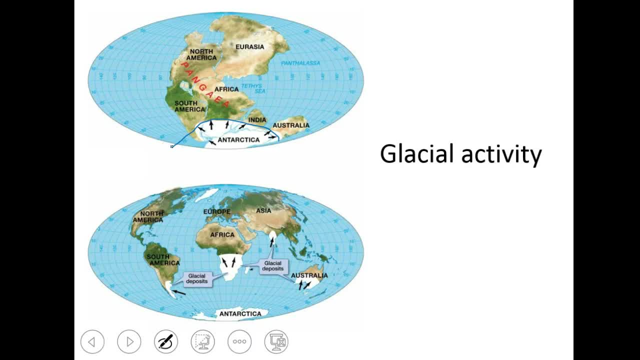 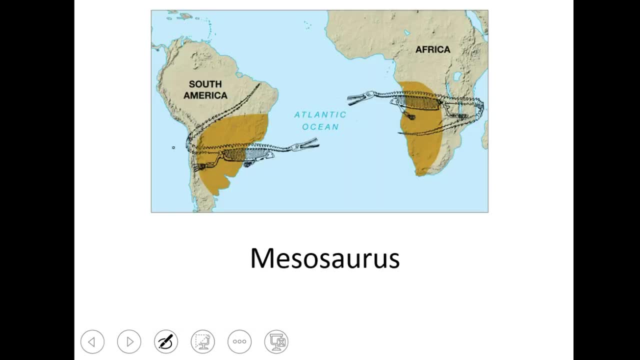 which suggested to him that these were in a much colder region of the Atlantic Ocean. So we've got mountains and glacial activity in what are now warm places- Very, very strange. And these gave him the clues about what fit together. And then, last but not least, the Mesasaurus are these big fossils that we find in South America and Africa. 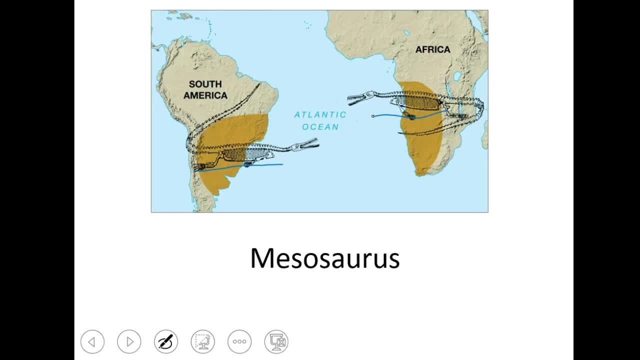 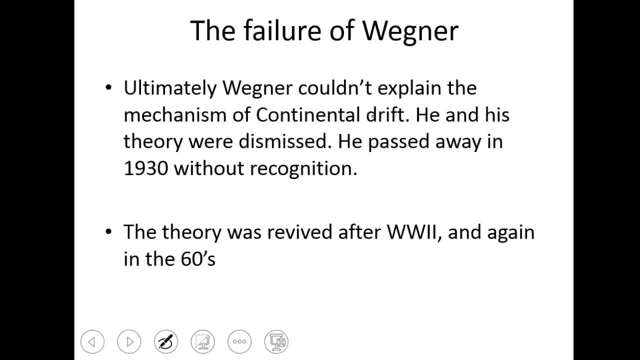 The exact same animal And it's incredibly unlikely that those developed independently of one another into the exact same animal, So again suggesting that they they occurred on a continent that was together. They occurred on a continent that was together. The failure of Wagner's hypothesis. 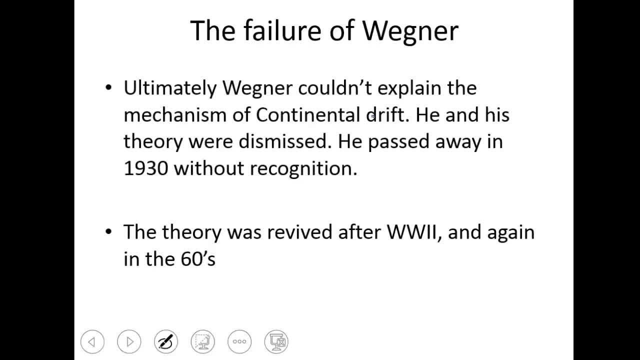 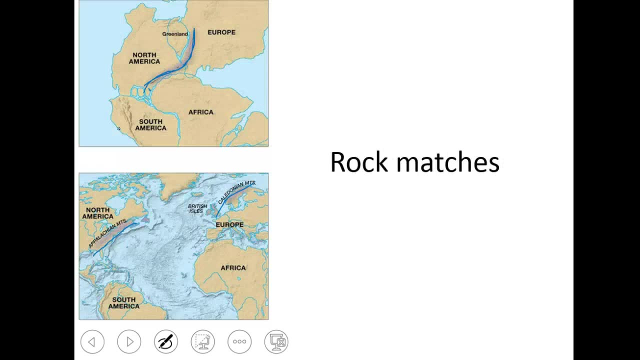 I mean, he had all this really great evidence and people still laughed him out of town. Ultimately, the failure of his whole hypothesis was that he couldn't explain how this was happening. He couldn't explain the mechanism behind continental drifts, And they would say, oh yeah, Alfred, all the continents used to be like this. 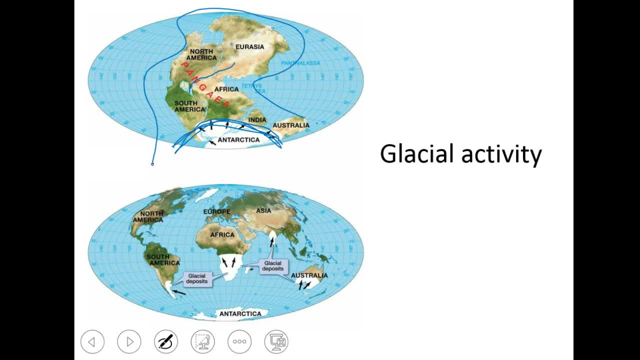 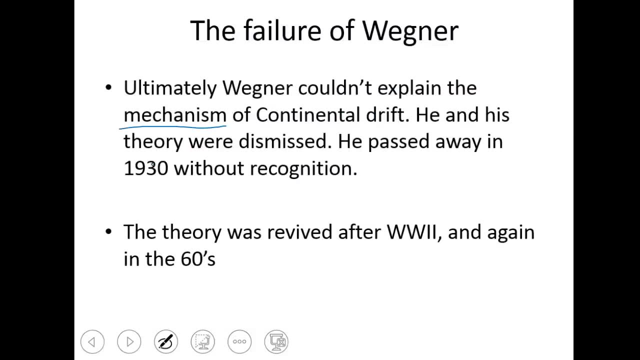 Well, how'd they get to where they are today? And he couldn't answer that Right. And because of that, because he couldn't tell them how it happened, they completely dismissed his theory. He passed away in 1930 without any recognition of that. 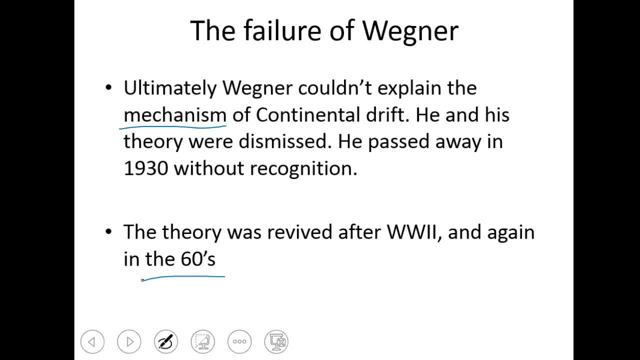 It wasn't until 1960, after World War Two- I'm sorry, It wasn't until right after World War Two- that evidence began to be collected, And then finally, in the 60s, the theory of plate tectonics was was created as a whole. 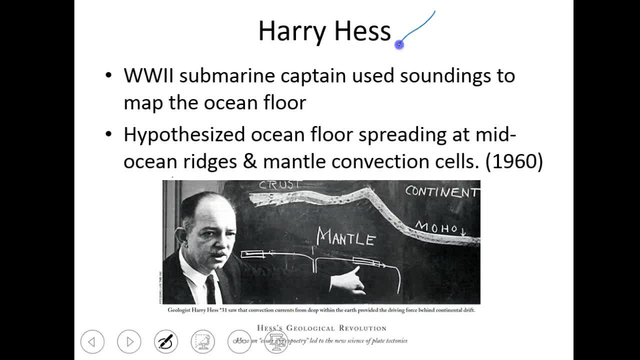 Harry Hess- another name that I want you to know- is responsible for the revival of the theory of continental drift. So he was a World War Two submarine captain, and they would use their radar or soundings to map the ocean floor. And so he realized when they were doing soundings, looking for other U-boats, that they were also mapping the ocean floor. 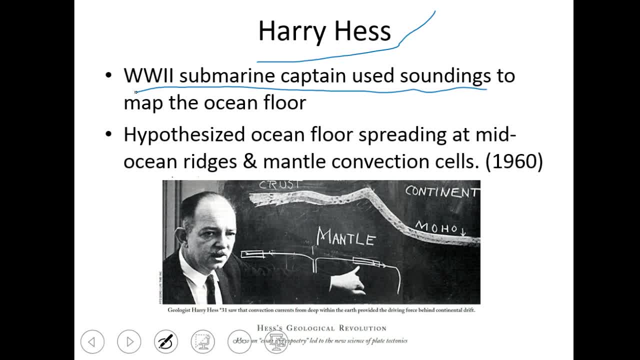 And he saw some really interesting things. He saw some really interesting things about there. He realized that in the middle of the Atlantic there's this huge mountain range that goes up and then there's a little dip in the middle and it goes up again and then back down into the abyss. 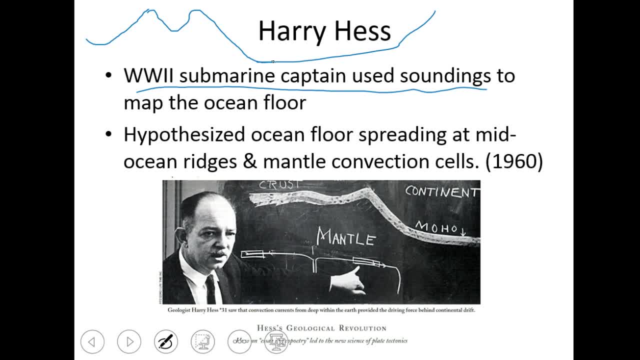 And he said, hmm, that's really odd. That looks like a lot, a lot like a valley right down in the ocean floor. So he actually hypothesized ocean floor spreading and mid-ocean ridges and mantle convection cells in 1960.. 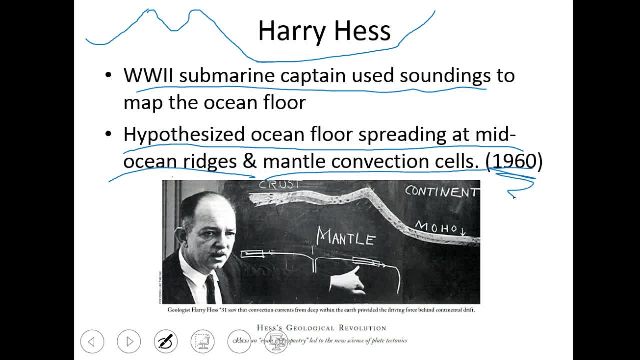 So he's the one that gave the how to continental drift. He answered that how? He said there's this big ridge in the middle of the ocean where mantle activity is coming up and creating new crust, And this is what's happening. That's why the Atlantic Ocean is getting better. 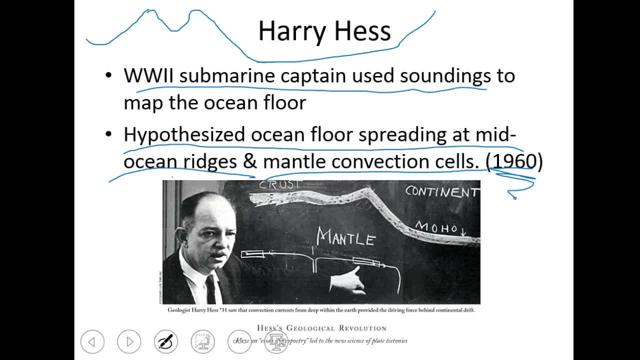 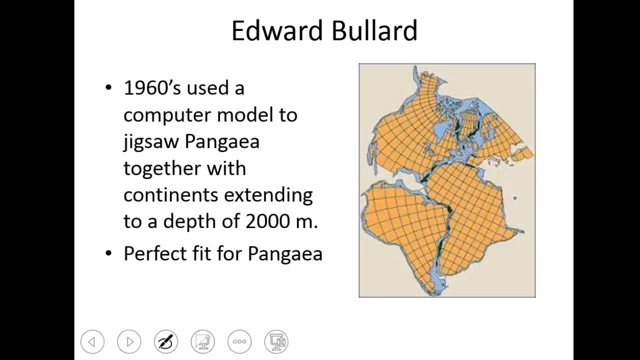 It explains why the continents are there now. And he proposed mantle convection cells as the, as the mechanism behind that Right. So in the 1960s, Edward Bullard, another scientist, actually used a computer model to jigsaw Pangea back together a little bit for the continental fit. 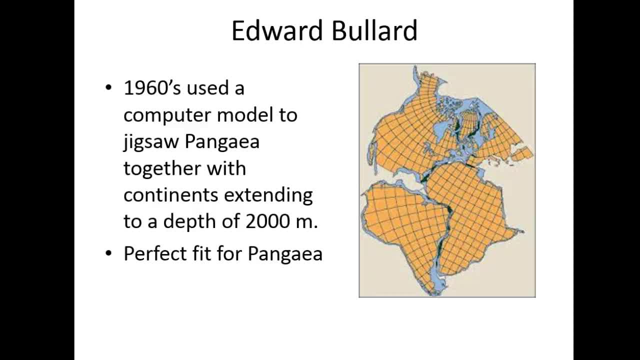 One of the problems that Alfred Wagner had was that the continents didn't fit perfectly together, And so what Edward did is he extended the margins of the continents to a depth of 2000 meters, which included included the continental shelves of those continents. Once he did that, he realized that this is what gave Pangea a perfect fit. 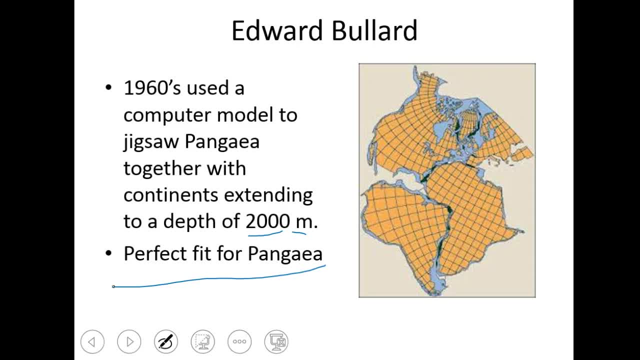 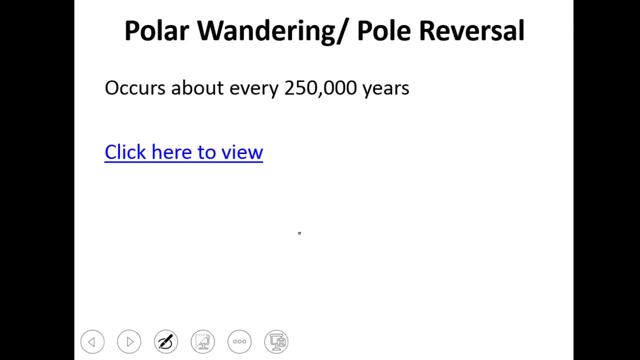 That in the past perhaps sea levels had risen and fallen such that that depth of what is now 2000 meters underwater might have once upon a time been above land. Polar wandering is another really good piece of evidence that kind of contributed to our understanding of Pangea. 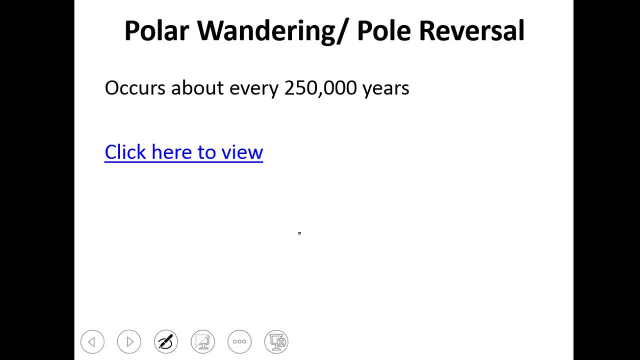 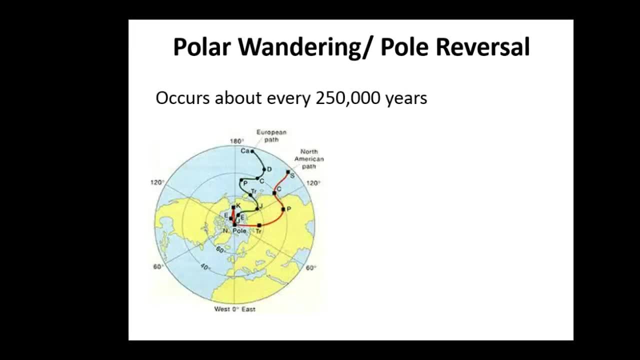 So we're going to go back to our understanding of continental drift and of plate tectonics. So what we see is that the actual magnetic North Pole- right that thing that gives us the declination on nautical charts, the actual magnetic North Pole- has wondered over time- and it's not always been by the geographic North Pole- that what we consider to be zero degrees. 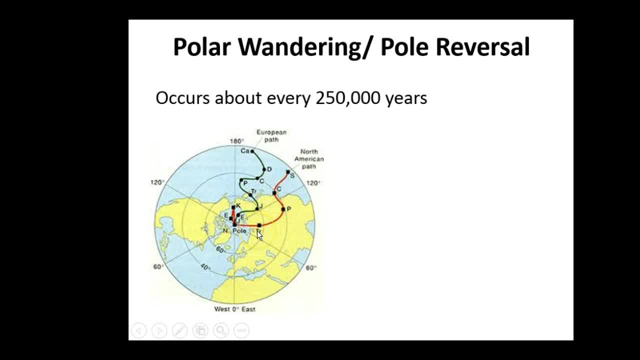 It changes, It changes, It changes all the time, And so with this, what we get is that as rocks are forming in the ocean, they record kind of the history of where this magnetic North Pole used to be, And about every 250,000 years or so, our Earth experiences a magnetic reversal. 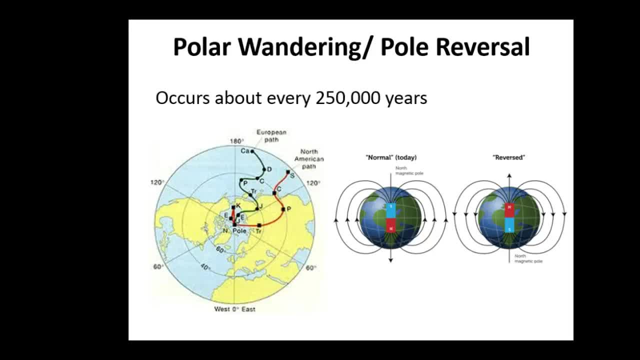 And I'm about to tell you how we know this. But what we consider as normal today has a magnetic south At geographic North Pole and a magnetic North Pole at our geographic South Pole. But again, we have records in the rocks that about every 250,000 years our magnetic field is exactly the opposite. 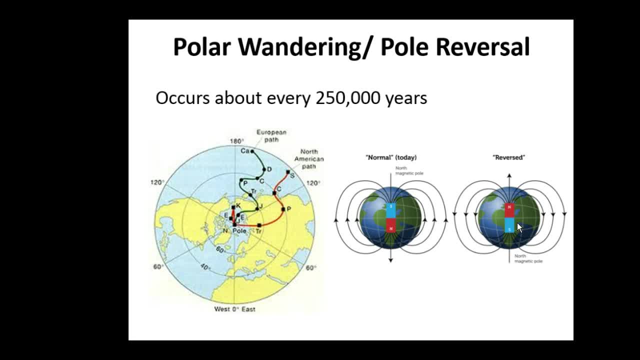 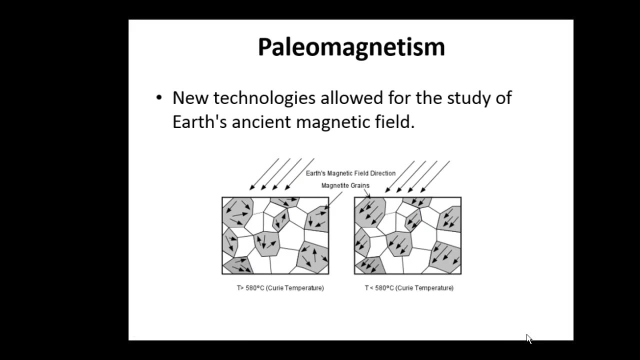 And so if we were around while a magnetic reversal happened, suddenly, all compasses would point towards the South Pole instead of the North Pole, Right. So what we see is called paleo magnetism, And so paleo magnetism is just. paleo means old. 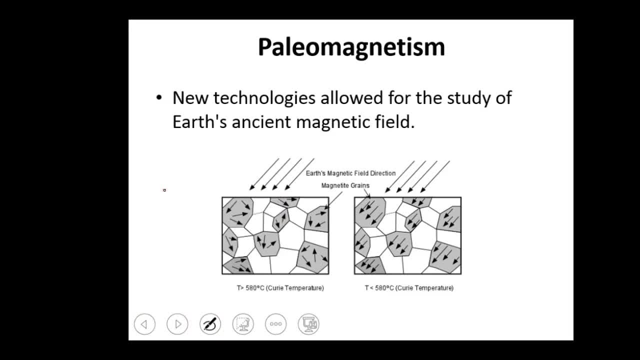 And as rocks form, they kind of form these tiny little bar magnets inside of them. So as magnetite, which is a mineral, cools, it orients itself in such a way as to become this little magnetized piece of mineral that points directly at Earth's magnetic field. 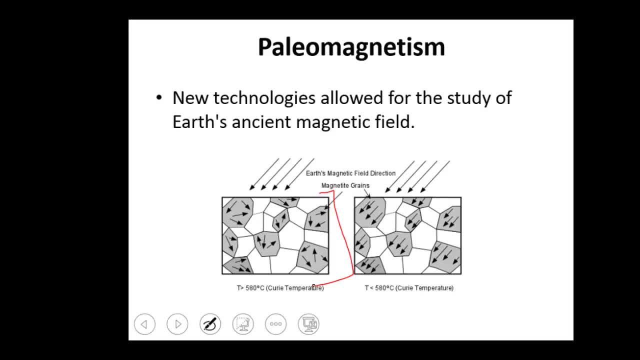 But once it's cooled and once it's formed into a rock, it doesn't change direction, And so there's a magnetic reversal. It's not like this suddenly orients itself towards the new magnetic pole. It's fixed it where the magnetic magnetic pole was when that rock turned into a rock: from liquid rock to to solid rock. 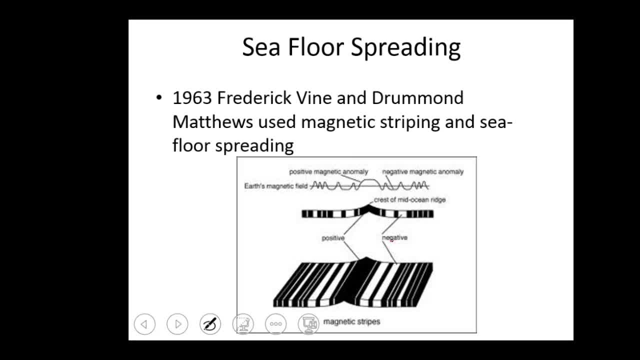 In 1963, Frederick Vine and Drummond Matthews used magnetic field. Matthews used magnetic striping in the sea floor to explain sea floor spreading, And so magnetic striping in the sea floor is at the mid-ocean ridge, where this liquid or plastic rock is coming up and forming new rock. 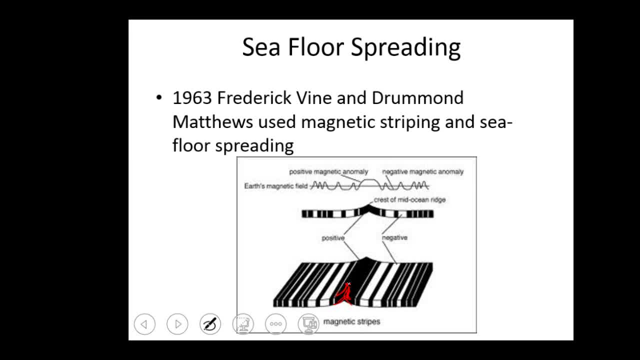 As that cools off, it orients itself towards the North Pole. But what we see as we go out into these older rocks is that some are saying North Pole is down here, Right, And we call these magnetic reversals. These are periods where the Earth's magnetic field was flipped. 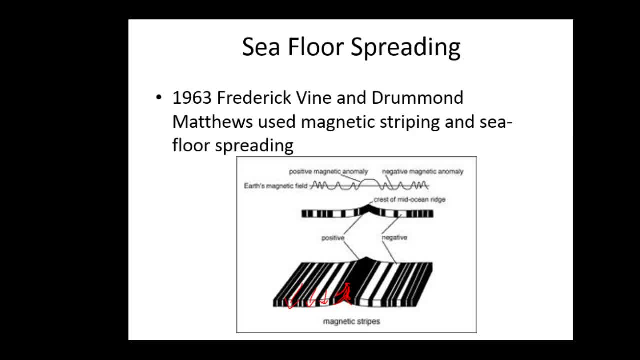 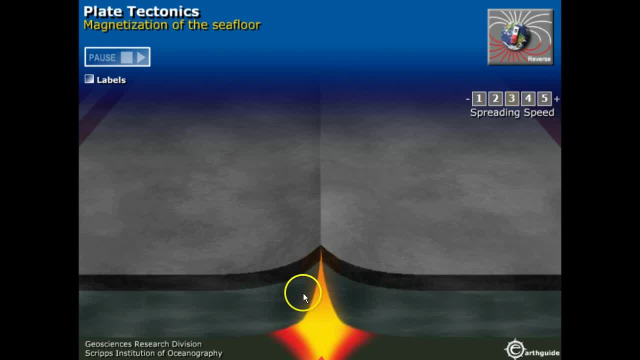 And I want to give you an idea of how all this happens. So I've got this, this little animation to do that And what we see is that we've got a spreading center, divergent boundary or something like the mid-Atlantic ridge, And it is that mantle plume is coming up and kind of pushing this lithosphere up. 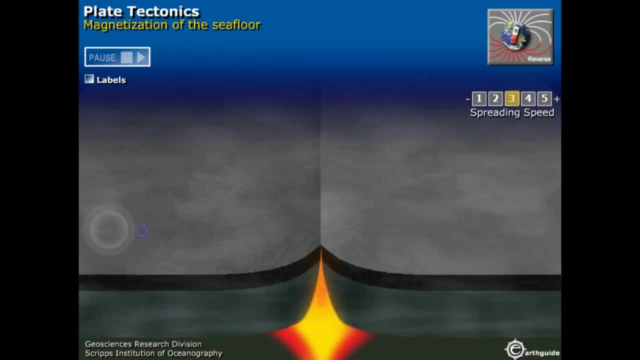 And you can see that here And it's it's spreading out and creating new ocean floor. I'm going to slow this spreading down a little bit, Maybe not that slow. There we go And I want to note that currently, in this magnetic floor, the magnetic field of the Earth is as we experience it today. 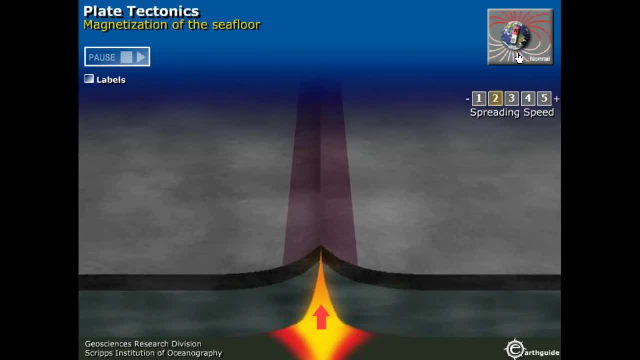 But if I reverse this magnetic field we get a region where rocks are cooling and saying that magnetic north is at geographic north. And then if I flip it again, Say it's been two hundred fifty thousand years, I start to get this kind of striped pattern on the ocean floor as I change the poles, as I reverse them. 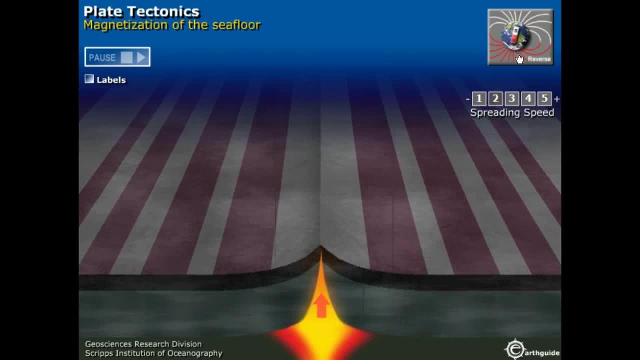 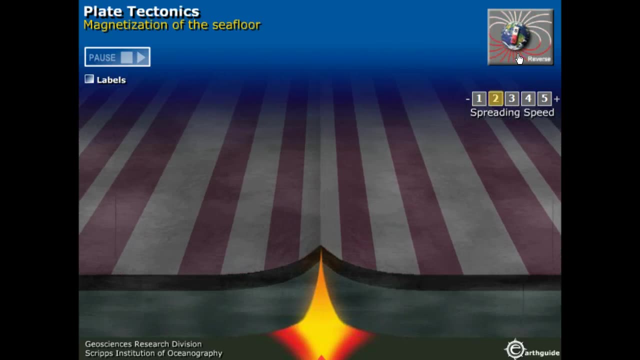 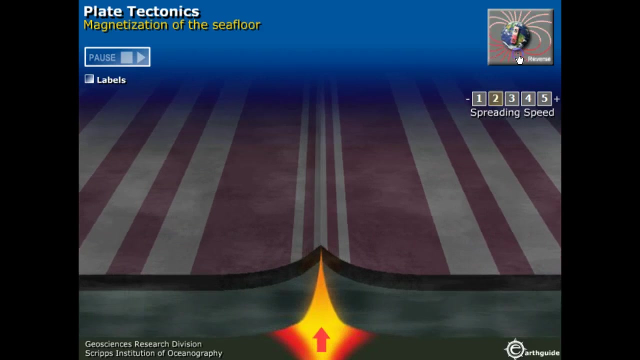 And so what we see is that about every two hundred fifty thousand years on the ocean floor we get a reversal, And that's on average. It's not consistently every two hundred fifty thousand years. Some are a little bit longer than others, And then there are periods where it might reverse very quickly. 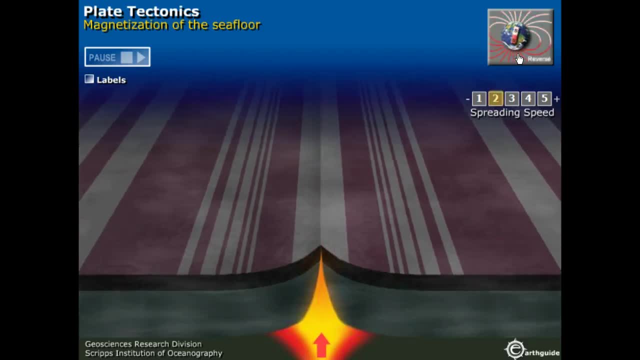 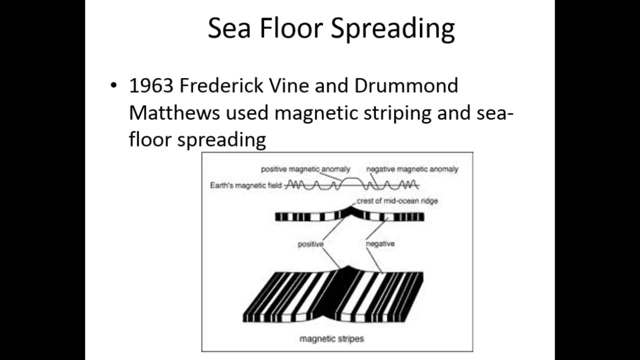 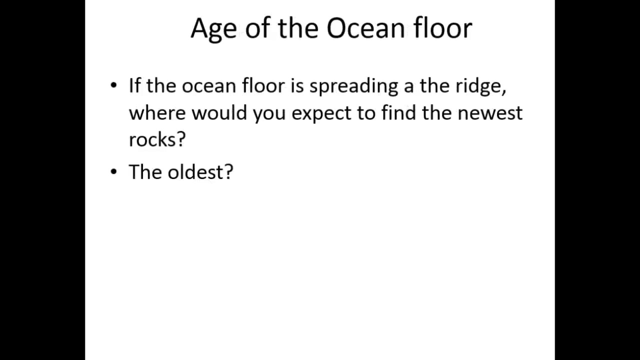 And we get shorter stripes and then maybe some longer ones. Right, But this is all recorded in the history of the ocean floor. So when in 1963, Frederick and Drummond began mapping the magnetic anomalies of the sea floor, this further supported seafloor spreading and further supported Harry Hesse's idea of plate tectonics and then the age of the ocean floor. 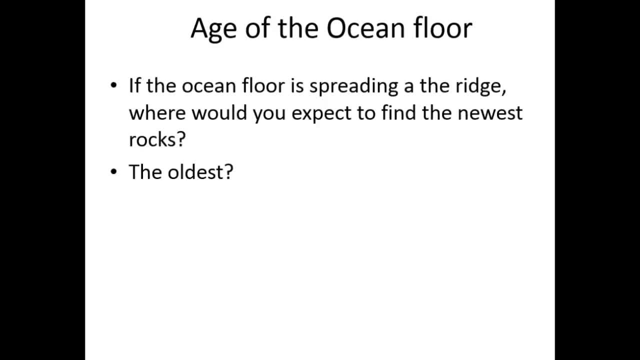 So if the ocean floor is spreading from the middle- in the Atlantic at least- then where would you expect to find the newest rocks? Well, right in the middle of the ocean, where they're being made, And then the oldest rocks would be towards the edge of the continents. 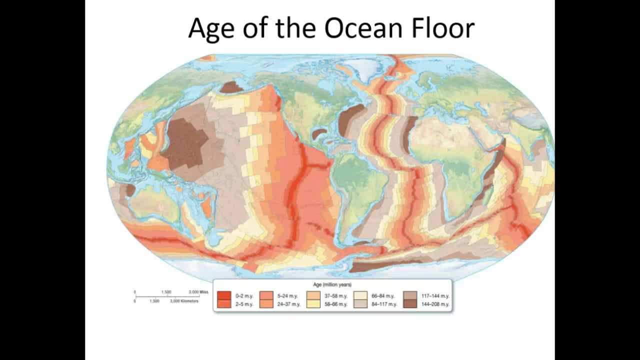 And we also find this to be true- that when we date those rocks, the newest ones are occurring along these spreading centers, So right down the middle of the Atlantic, And then we've got spreading centers all over the world. We've got some over here where we find very, very young rocks. 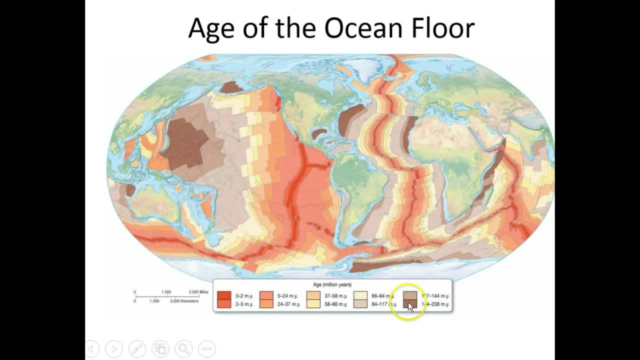 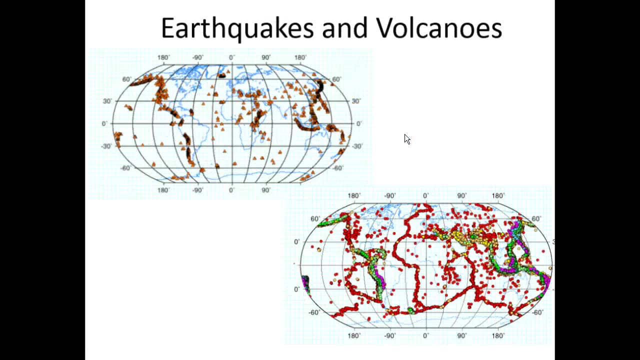 And then the oldest rocks in the world Are one hundred and forty four to two hundred and eight million years old, And they're right along the edges of these continents from when they used to be together. And that's the oldest rocks in the sea floor- by the way, not the oldest rocks that we have on Earth. 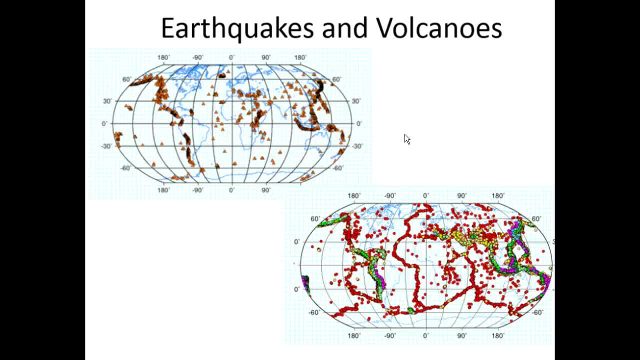 The other thing that we find is that earthquakes and volcanoes are intimately related with with plate tectonics, And so this is a map showing the volcanoes of the world in the upper left And earthquakes of the world in the lower, lower right.